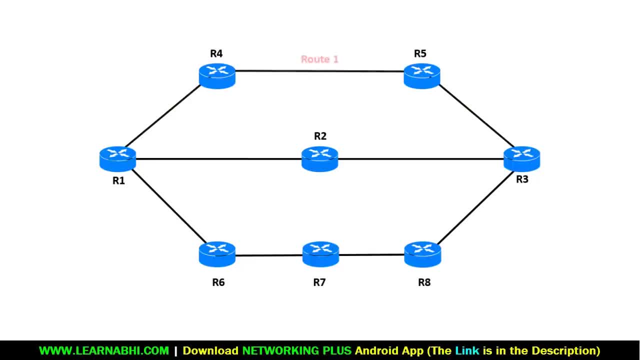 Here we have three possible routes: route 1,, route 2, and the route 3.. And the RIP will choose the second route because it has only two hope counts, whereas the route number 1 has three hope count and the route number 3 has four hope counts. 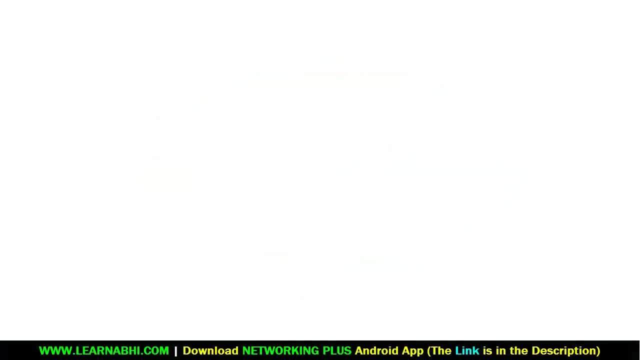 Let's take an another example. There are six routers connected in the network, where router 1 wants to send data to router 4.. Here we have two possible routes to reach the destination, that is, route number 1 and the route number 2.. But in this scenario both the routes have the same number of hope counts, that is 3.. 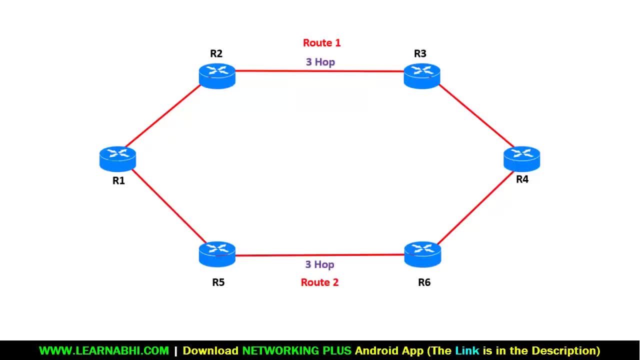 Now can you tell me which route does the router 3 follow RIP is going to choose for sending the packets? The router will send the packets via both the routes at the same time And like this it is going to manage the load balancing and the data will reach to the destination bit faster. 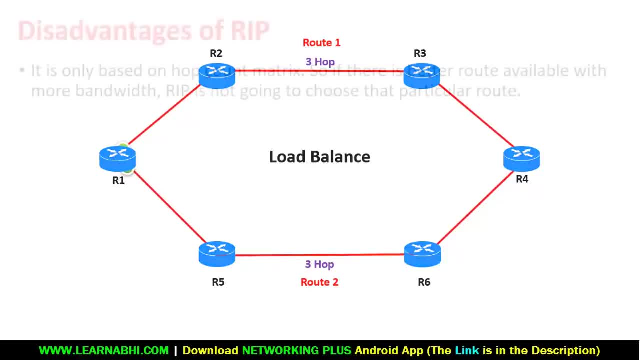 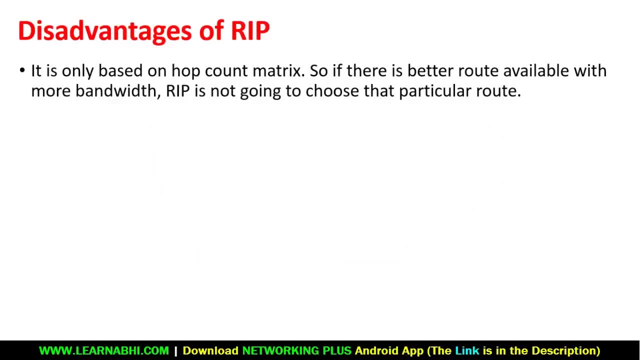 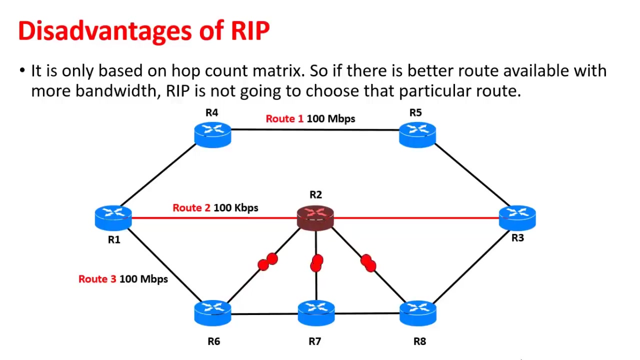 Now let's look at the few disadvantages of RIP, that is, Routing Information Protocol. RIP is only based on hope count matrix. So if there is a better route available with more bandwidth, RIP is not going to choose that particular route, As, for example, there are eight routers connected in the network where route with the least number of hope is route 2.. 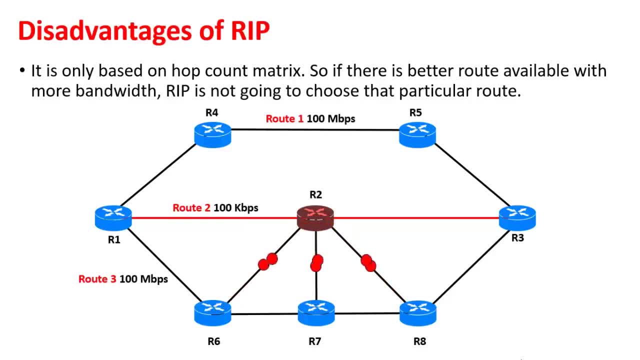 But there is lots of traffic in this particular route. In this case the router is not going to check that. route 1 is free. So if there is better route available with more bandwidth, RIP is not going to choose that particular route. 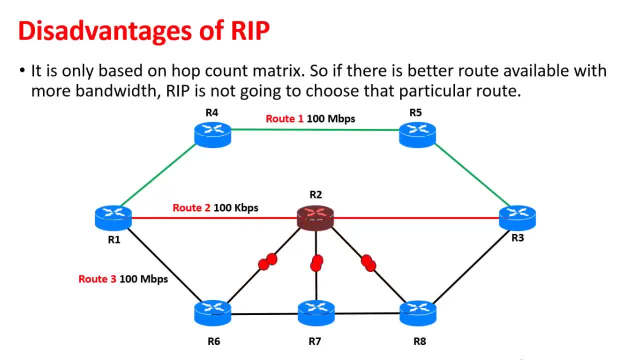 And data can be reached faster. Instead of this, it will send the data via route 2 only, and this particular route will become more slower due to heavy traffic. So this is one of the biggest disadvantages of RIP. Now let's look at the few more disadvantages of RIP. 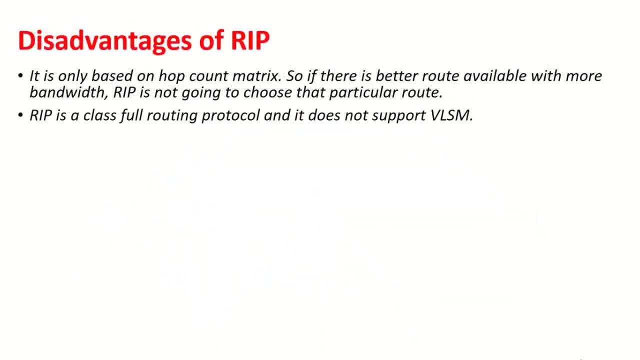 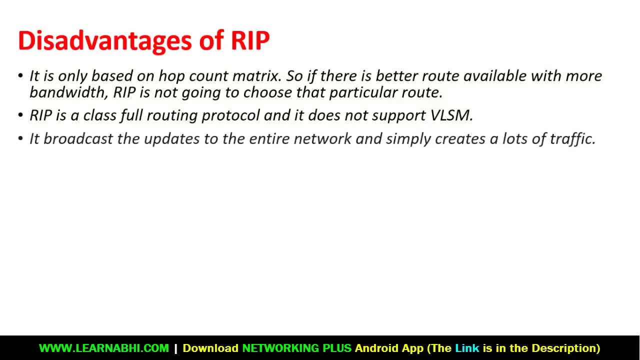 That is. RIP is a class full routing protocol And it does not support VLSM. That is VLSM. That is VLSM. As you can see, the RIP G subdivision is built into a variable length subnet mask. 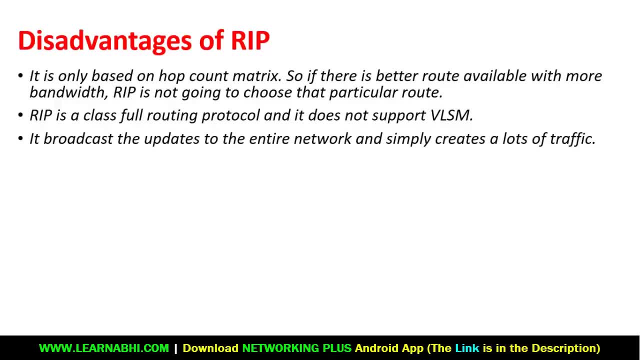 RIP broadcasts the updates to the entire network and simply creates a lot of traffic. Bandwidth utilization in RIP is very high, as it broadcasts its updates every 30 seconds. RIP supports a maximum of 15 Hоп counts, Which mean maximum 16 routers can be configured in RIP, not more than that. 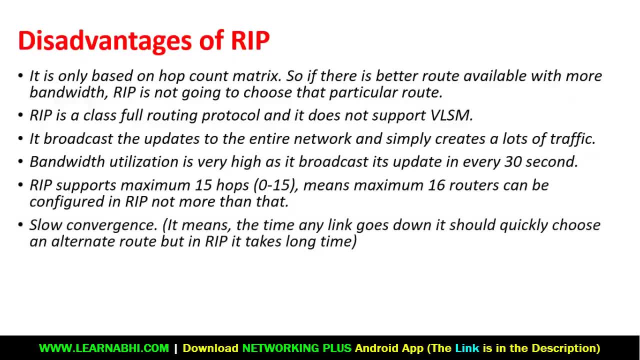 here the convergence rate is slow, which means the time any link goes down it should quickly choose an alternate route, but in case of rip it takes long time. the rib administrative distance is 120, which is also called ed value. the less ed value is more reliable, but the rib has the highest. 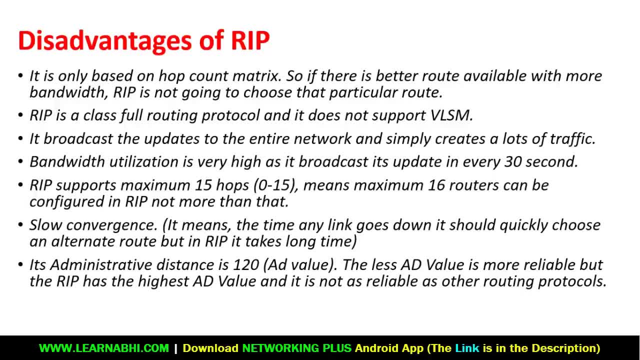 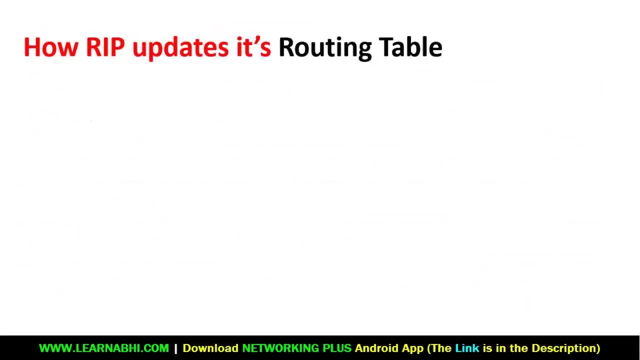 ed value and it is not as reliable as other routing protocol. now let's have a look how rip updates its routing table. rip update timer is 30 second. all the routers configured with rip send their updates in every 30 second. the rib invalid timer is 180 second, which means if any of the 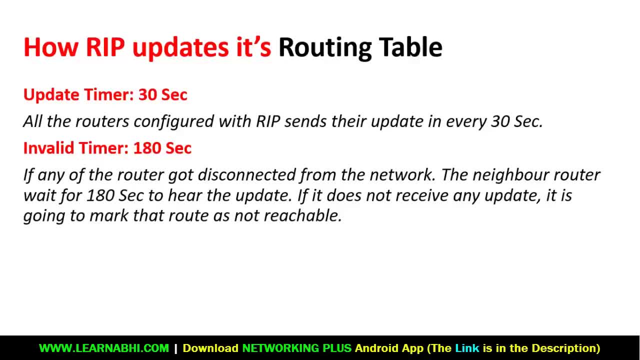 router got disconnected from the network or the link goes down the neighbor router. wait for 180 second to hear the update. if it does not receive any update, it is going to mark that particular route as not reachable. after that there is a flash timer which is 240 second. if the route does not go up or not send the update. 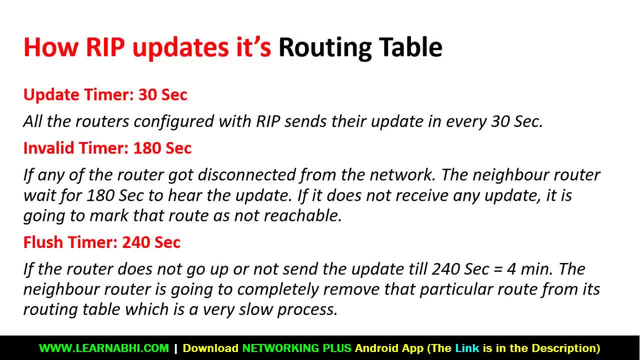 till 240 second, which is almost equal to 4 minute. the neighbor router is going to completely remove that particular route from its routing table, which is a very slow process. it should not take four minutes, guys. four minutes is too long time. as we noted, there are lots of disadvantages in RIP. 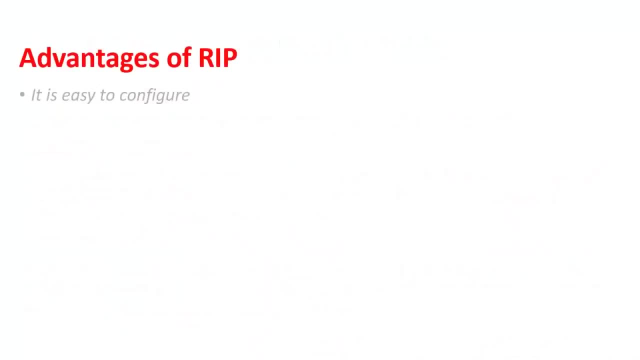 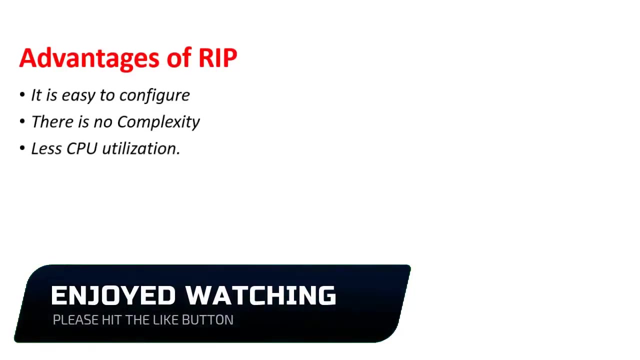 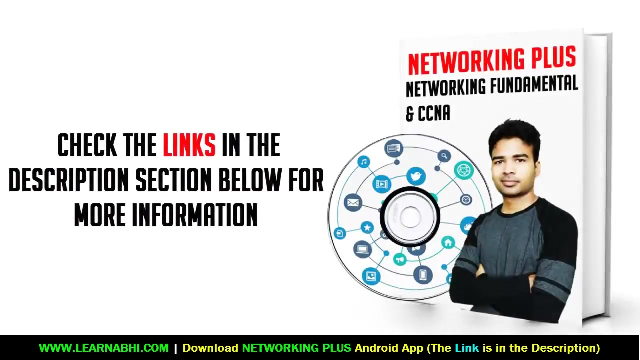 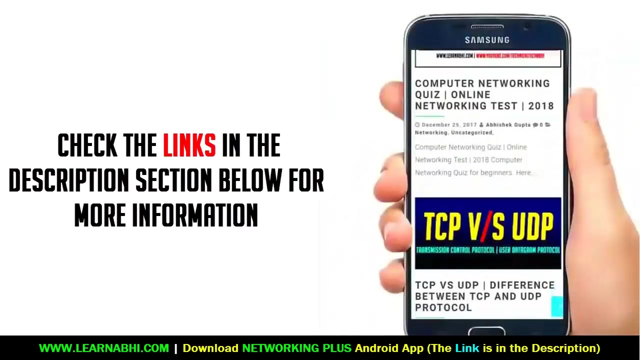 but here are few advantages too, that is, it is easy to configure, there is no complexity and the less CPU utilization. so, guys, this is the theory part of RIP, that is, routing information protocol. in my next video, I am going to explain you how to configure RIP in a computer network. so, guys, whatever things I have,